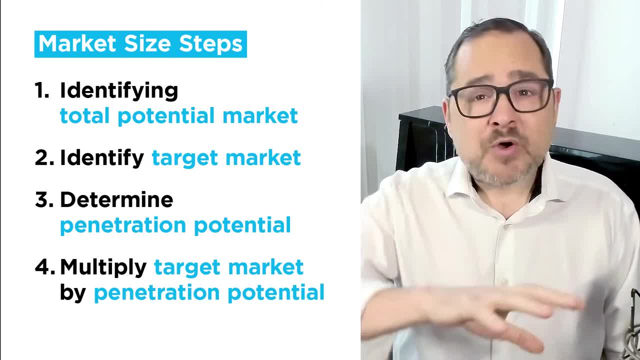 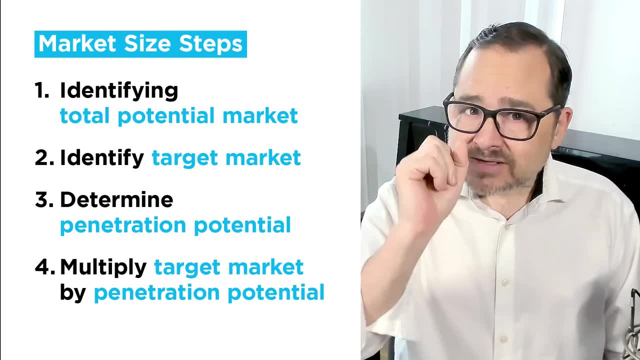 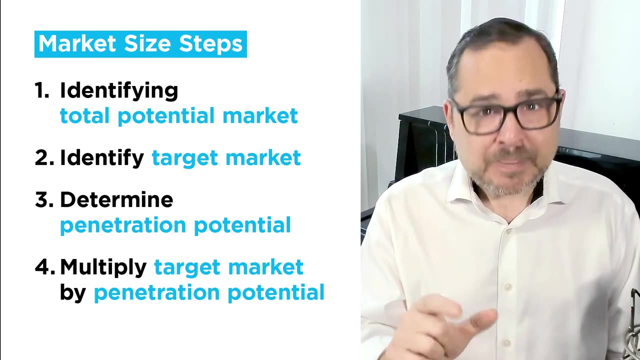 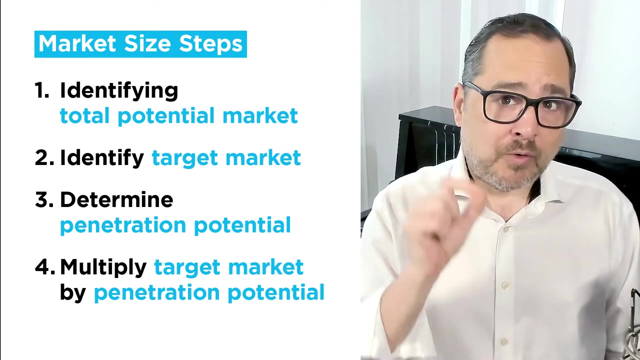 Then figure out your target. Take your target market within the TAM, And this can vary depending on geography and other factors. Next, take your target market and determine the penetration potential. Then multiply the target market by the penetration rate to find out your market size. 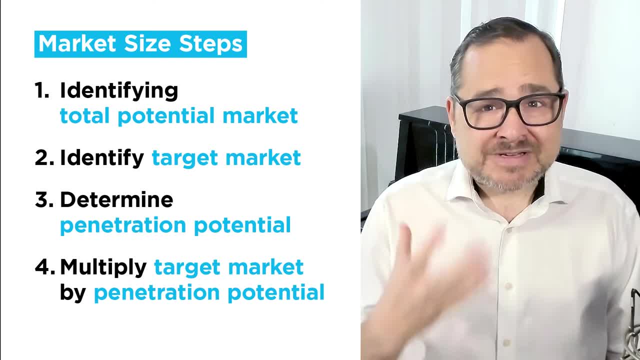 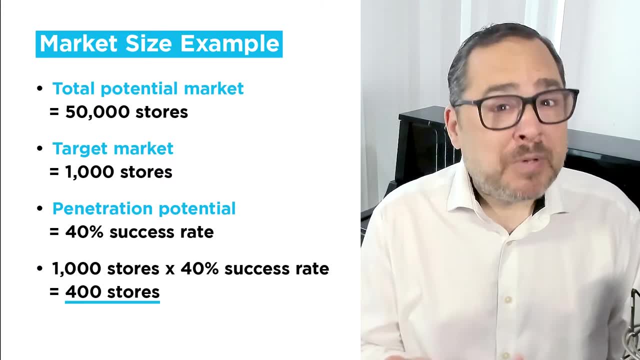 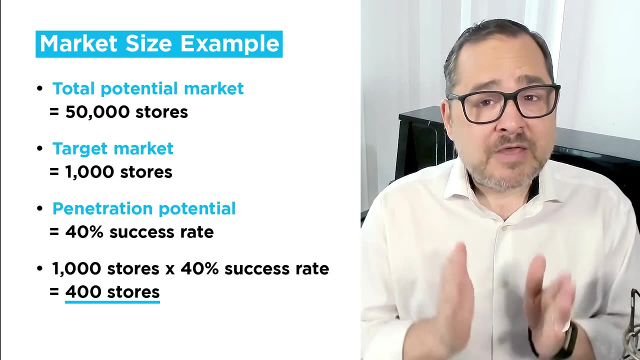 So likely. this isn't going to make much sense without a concrete example. So here we go. Let's say that you're selling picture frames and you want to calculate your market size. Again, first identify the total potential market in your country or TAM. 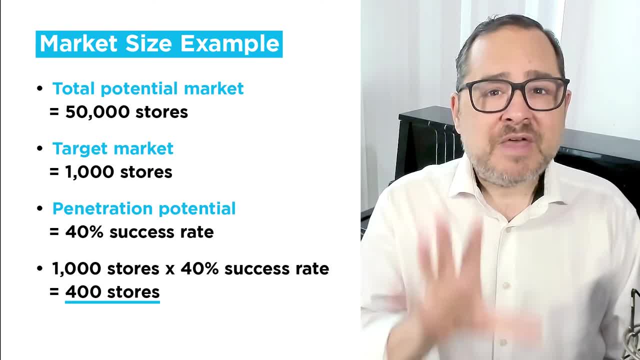 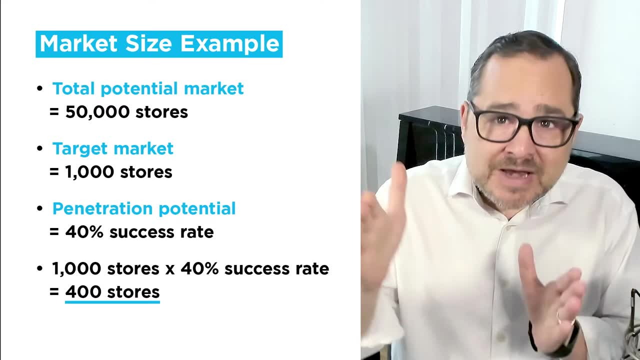 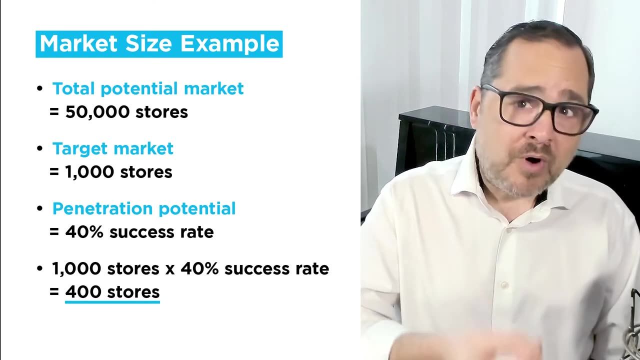 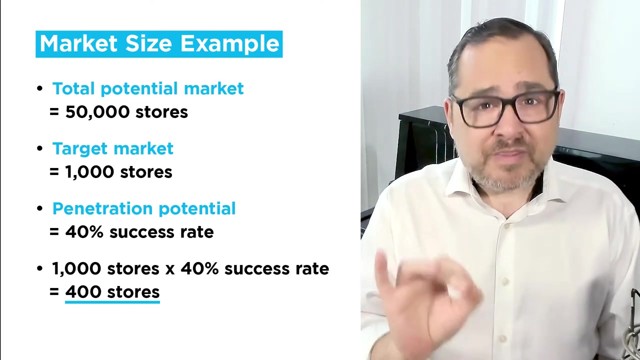 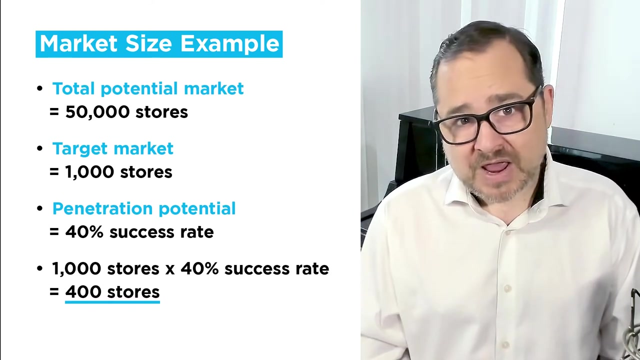 Let's say there are a total of 50,000 stores that might carry your product nationwide. Next, you narrow in on your target market. So say you only want to target certain states or provinces in your country. So of the 50,000, there are 1,000 stores that could carry your picture frames in specific geographical areas. 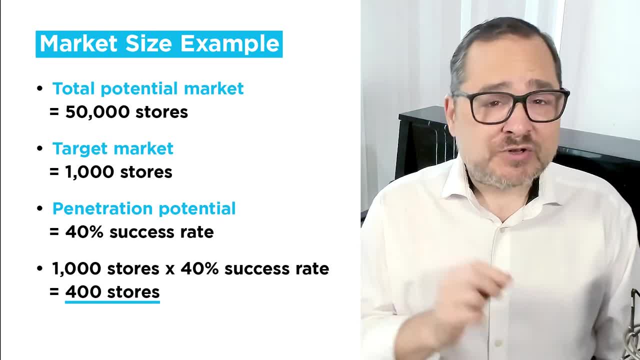 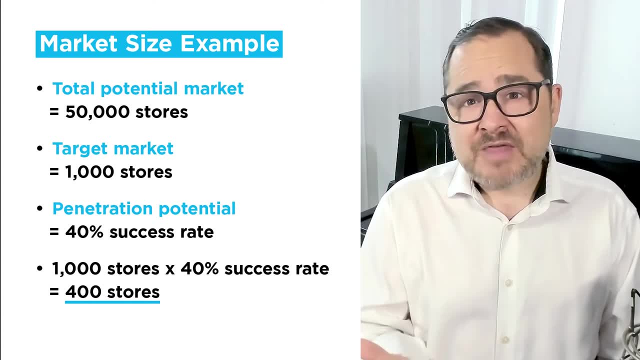 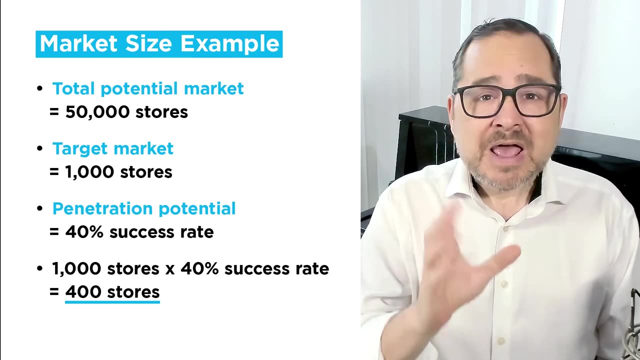 Next comes your penetration potential. So you do some research, speaking with different store owners, and you find that you will have about a 40% success rate for distribution. Now let's calculate: If we take the 1,000 stores times 40% success rate, you get a total of 400 picture frame stores. This is your market size. Now, if you want to figure out your market value or potential revenue, first determine the approximate sales For each store. we'll say you project $20,000 per year, And that's for each store. Then simply calculate: 400 stores times 20,000 equals $8 million. 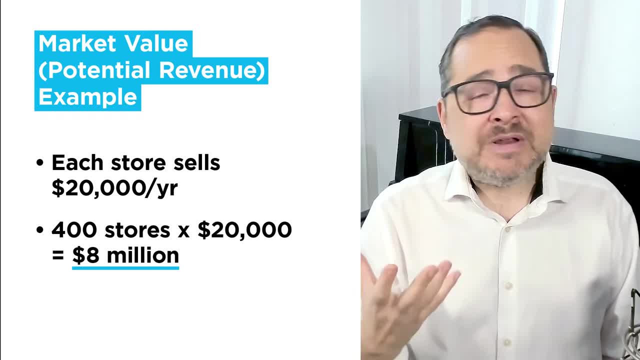 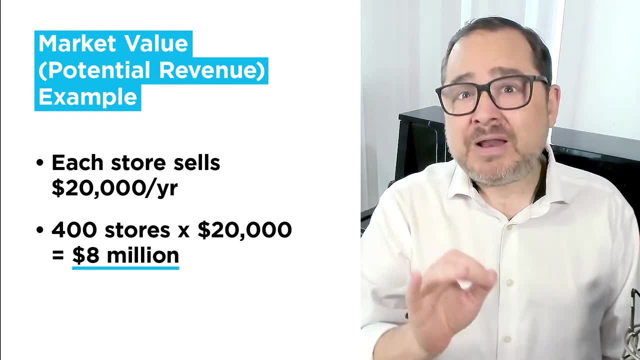 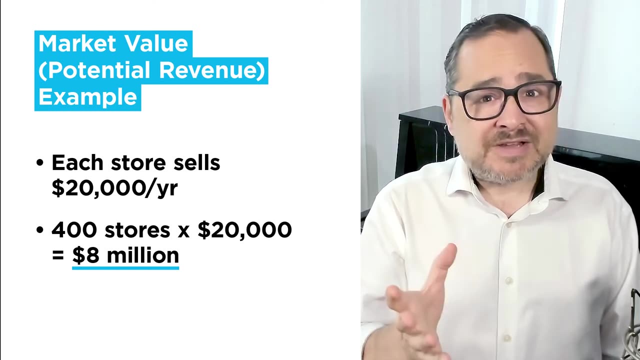 And that's it. Remember that this doesn't fully take into account your competitors, who may also be selling picture frames, and the fluctuations in the market, But it will give you a rough idea of potential revenue And what money remains for other initiatives, such as your marketing campaign. 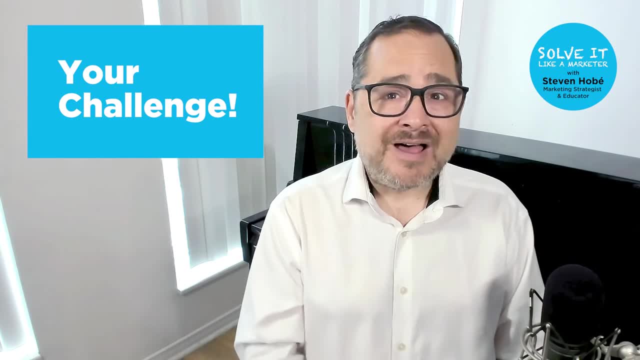 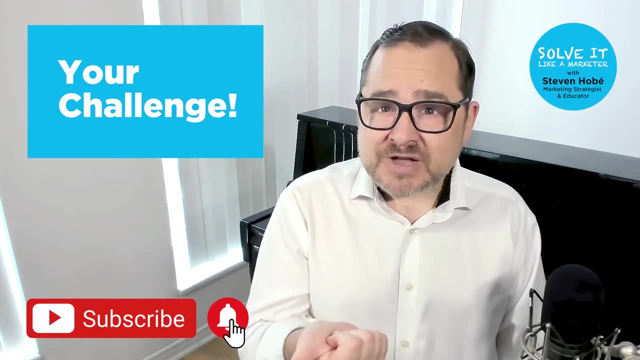 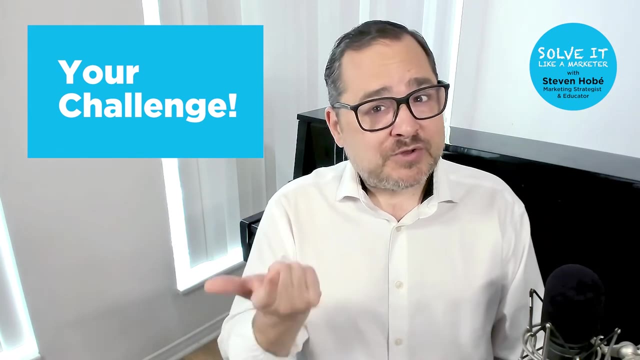 Okay, so you have your estimated market size. Now what, Well, market size helps your business? answer the following questions: How much potential revenue can you earn from this particular market? Is the market big enough Or do you need to adjust the target market?